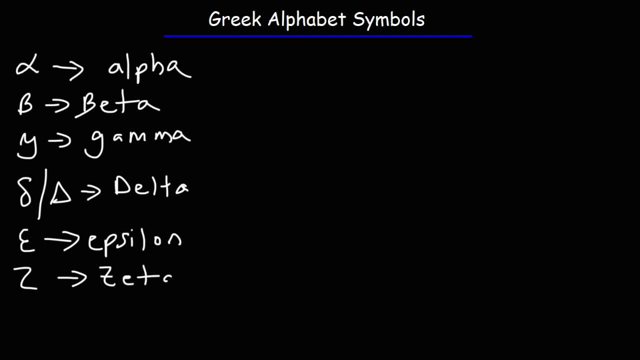 Next we have is zeta and phi physics. this would be impedance, particularly in an RLC circuit. the next Greek symbol is theta. now, I'm sure you've encountered this symbol if you you've taken a trigonometry or precalculus, so this would represent the. 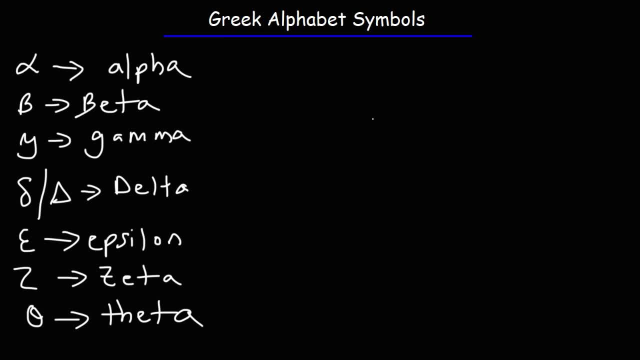 angle in trig. the next symbol is kappa, and this one. you've seen it in chemistry or physics. this is a lambda. in chemistry, this would be the wavelength of a wave, and the same is true in physics. next, we have this symbol, mu, and you've seen this. 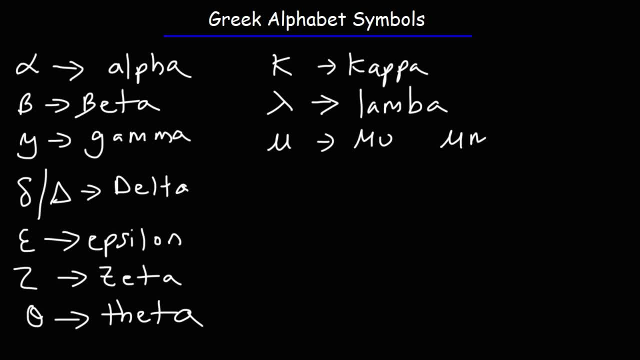 in terms of units. think of micrometers or micrograms. next, we have the Greek symbol nu, which looks like a V. this represents frequency when dealing with waves. the next one is pi, which is typically encountered in math and geometry. this is the value 3.14159 with 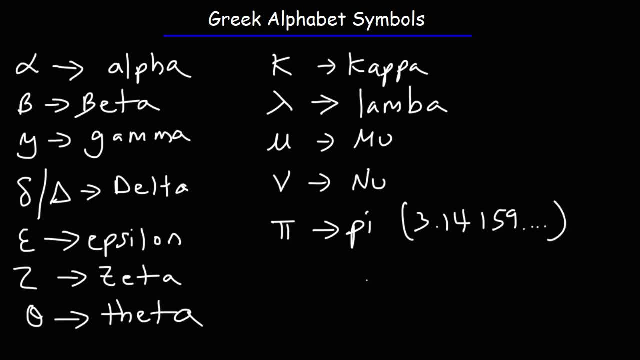 some other numbers after that. this is the value 3.14159, with some other numbers after that. this is the value 3.14159, with some other numbers after that. this added to that as well. in physics we have the Greek symbol Rho, which in 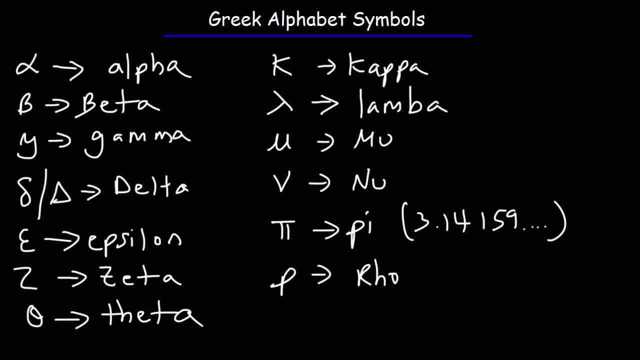 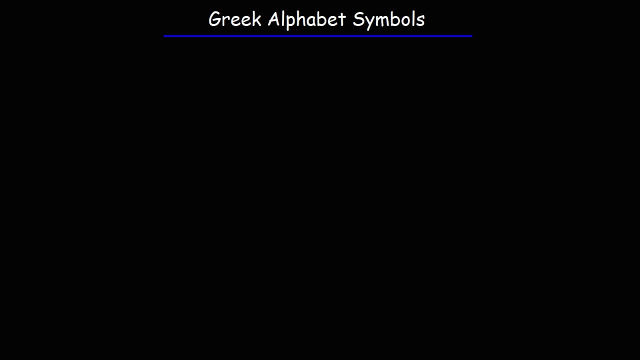 electricity topics, this would be resistivity, but in more classical physics, like, let's say, fluid mechanics, you might see this as density. now, since I'm running out of space, I'm gonna clear away a few things. now. the next symbol is sigma, which you'll see it in two forms: that's the lowercase of Sigma and this: 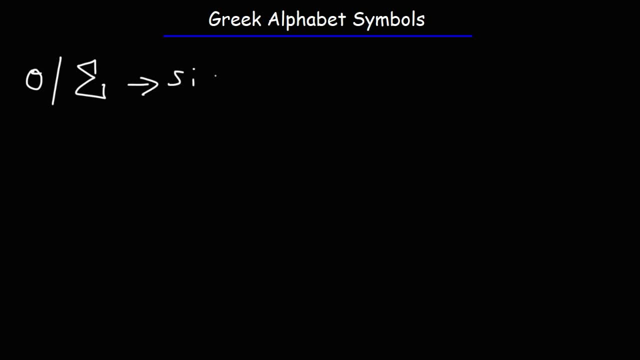 is the uppercase aversion of Sigma, so the lowercase Sigma. this will typically correspond to an angle, just as theta would represent an angle in trigonometry. the uppercase aversion of Sigma this is- you'll see this in math- this represents some summation or some. so, for instance, let's say, if we have the Sigma of x squared,